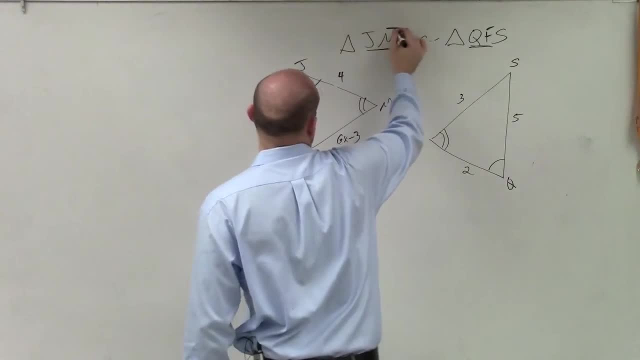 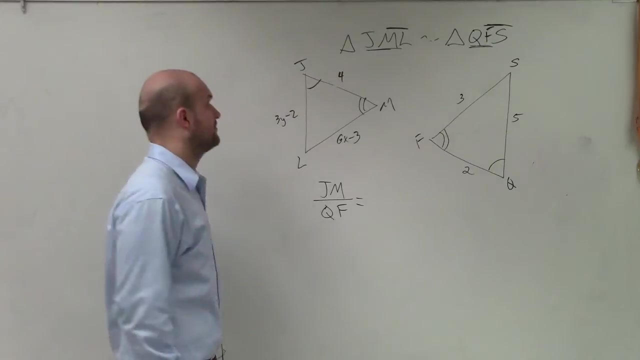 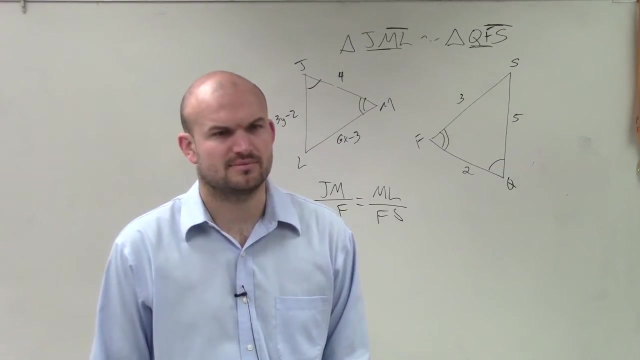 OK, OK, OK, OK, Which is equal to the ratio of ML. Then just walk around that way. ML relates to Fs. What is that On the ground? Yeah, Then that blue. Oh, your phone. You dropped your phone. 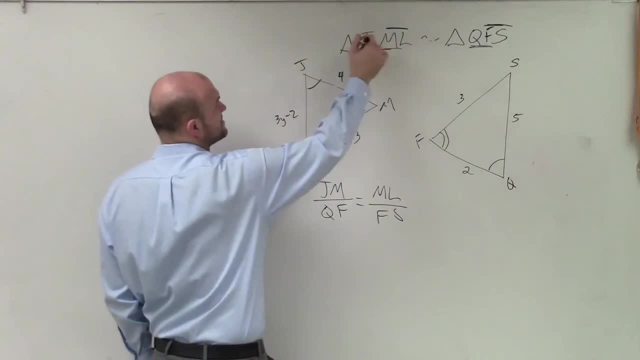 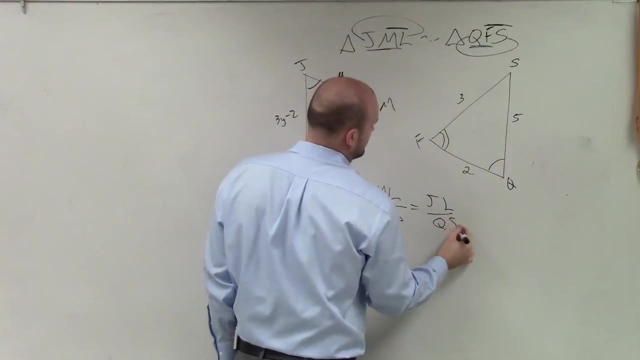 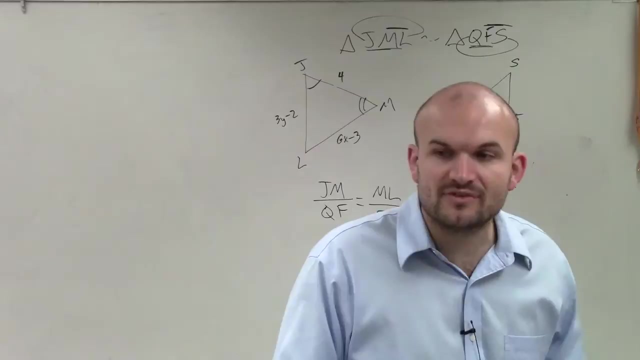 So ML relates to Fs And then JL relates to Qs. OK, So what I want to do now, ladies and gentlemen, is now I've taken my ratios, or I've taken all the side lengths and I've compared them to their other side. 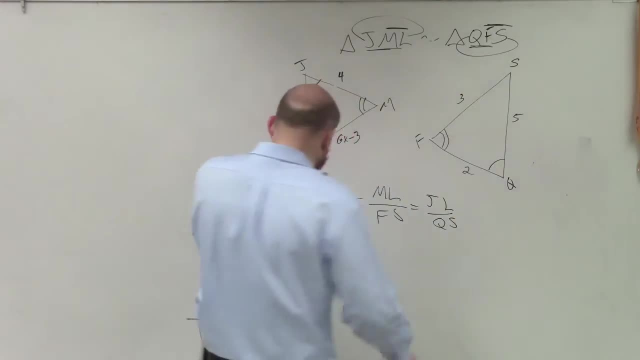 length of the other triangle. Now, if I want to solve for x, what I want to do is determine what is the one ratio where I know both of the side lengths. So JM, right, compared to QF. Do I have no variables here, right? 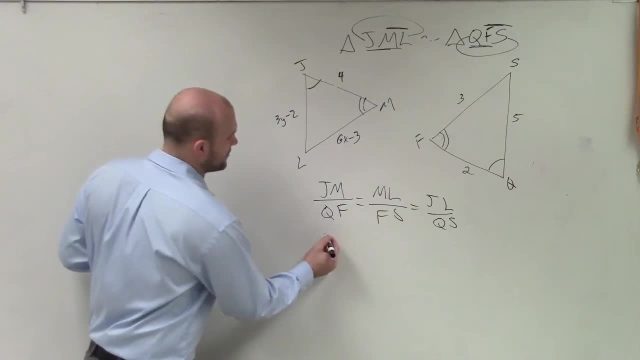 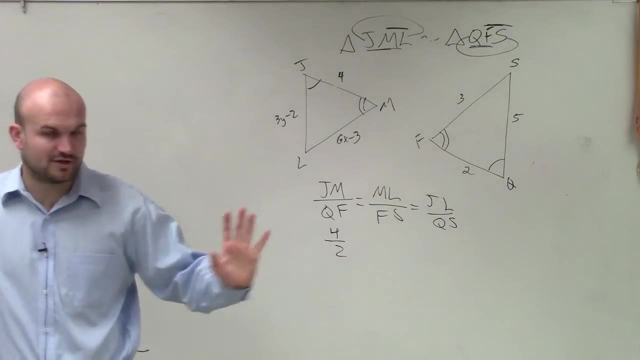 Do you guys agree? So therefore, I can say that JM is 4 is to 2.. OK, Now I'm going to leave it as that. I know you can divide the 2 into there, but let's leave it as 4 is to 2.. 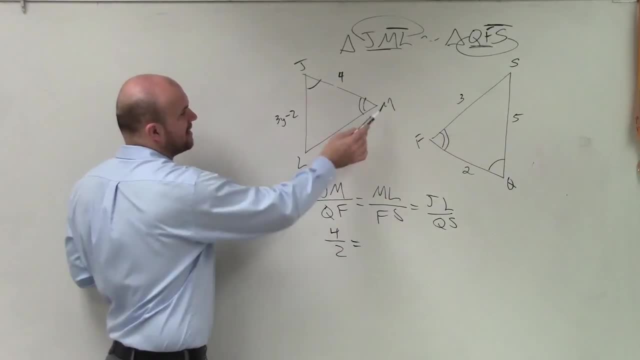 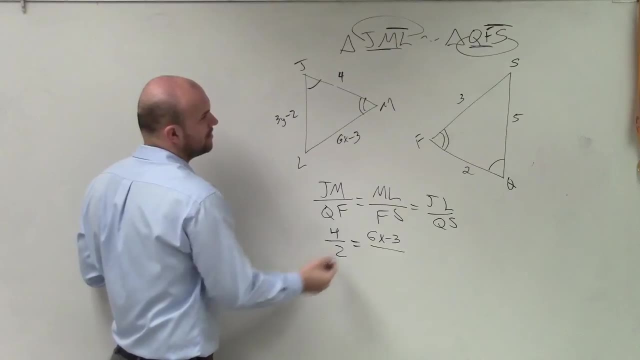 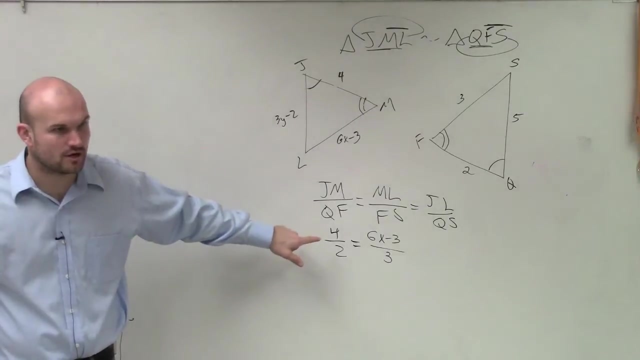 The next one: ML is to Fs, ML is to Fs. ML is 6x minus 3 over Fs, which is 3.. Can I solve this equation now, as it is, by using what we did last night in our homework? 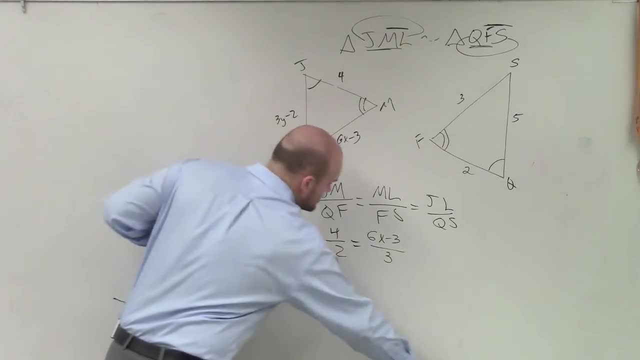 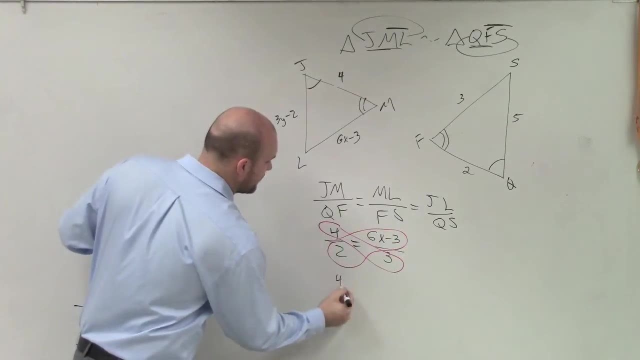 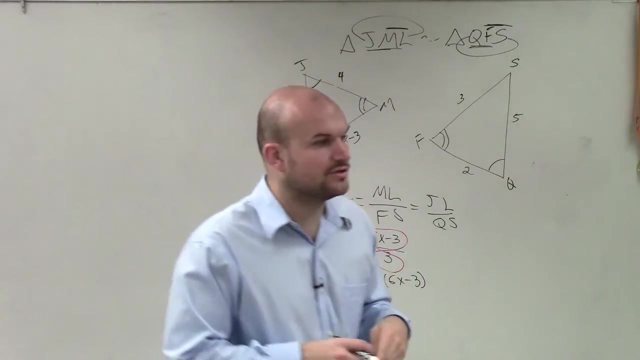 Yeah, Right, We can now apply our cross products. So now I can say: 4 times 3 is equal to 2 times 6x minus 3.. OK, Now I had a student that said: ah, I didn't know what to do when you had that binomial. 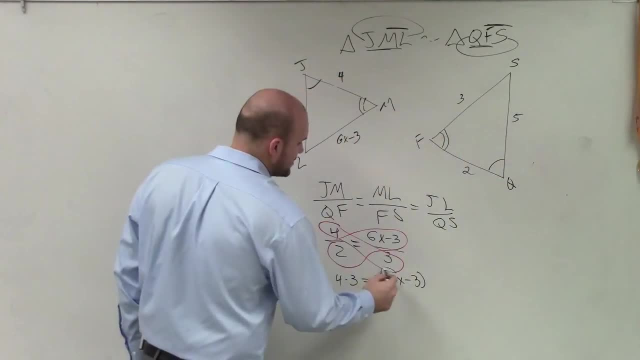 When you have the binomial, we need to be very careful and make sure that we apply distributive property. So therefore, I have 4 times 3, which is 12, equals 12x, minus 6, add 6, and I get 18 equals 12x. 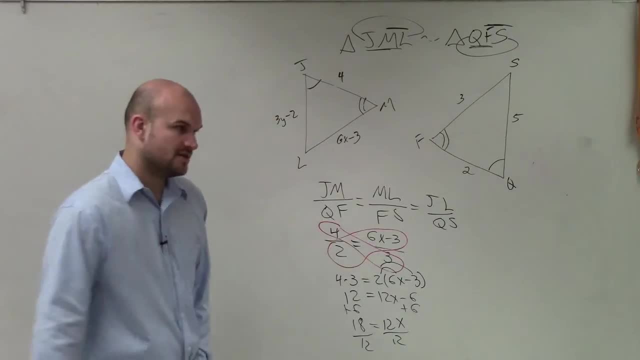 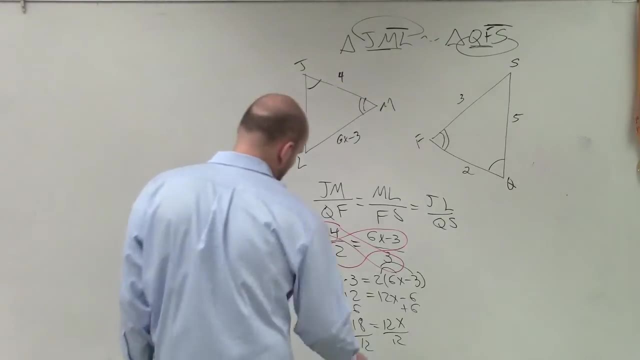 Divide by 12. That's going to be 1 and 1, 1⁄2 or 1.5.. OK, You can leave it as a fractional form as well. 1 1⁄2 or 1.5 is the same thing as a reduced fraction. 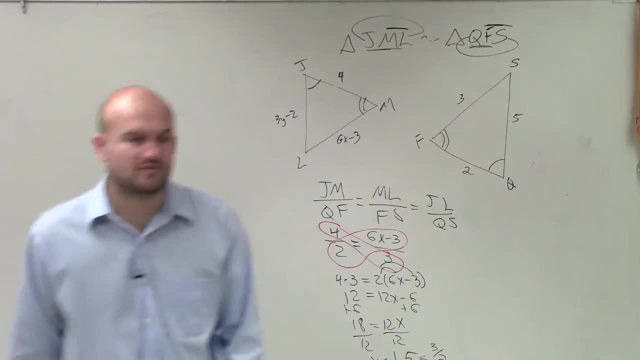 form of 3 1⁄2, which I would actually prefer would be 3 1⁄2.. So now We've got these two. Now I need to find JL and QS. I'm actually going to write it over here. 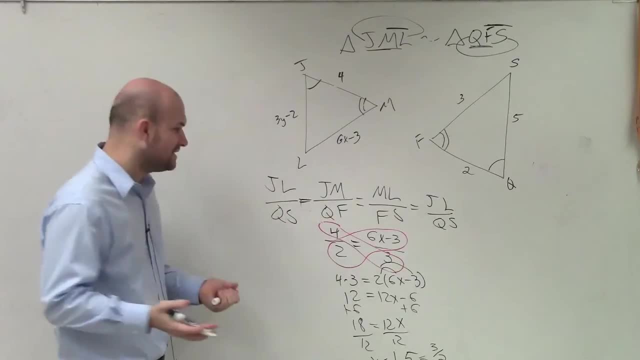 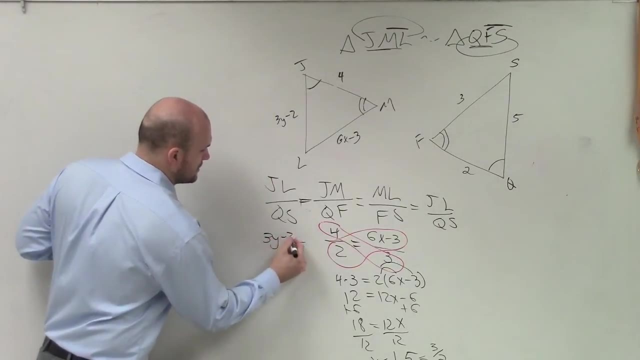 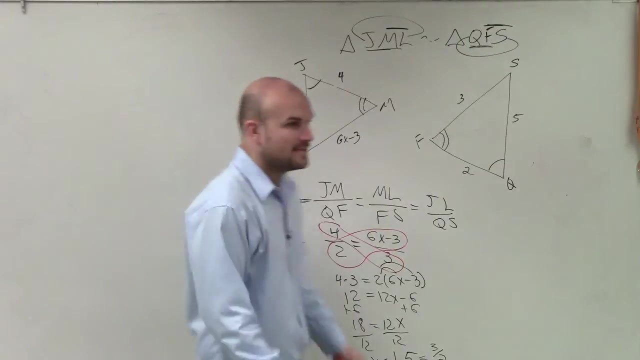 JL over QS. The reason being, ladies and gentlemen, is what's JL? JL is 3y minus 2. And QS is 5.. OK, So if I write my proportion over here now, I can do again cross multiplication again. 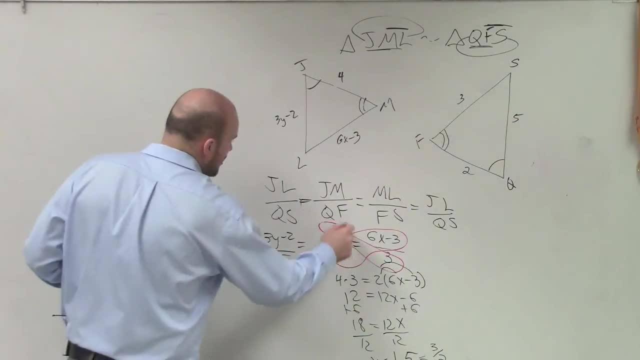 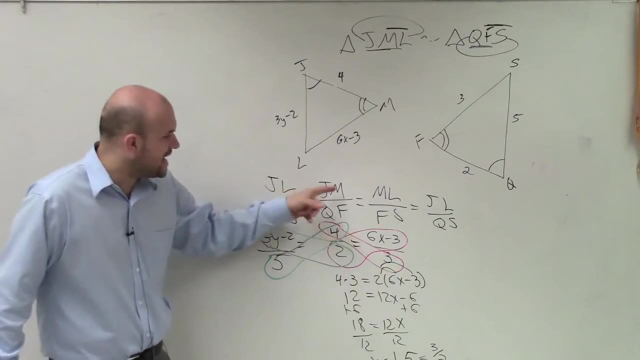 But what I want you guys to notice, what's so important about this, is notice which ratio I'm doing cross multiplication with twice. I'm doing it with the ratio JM and QF. What is the difference about this ratio JM and QF? 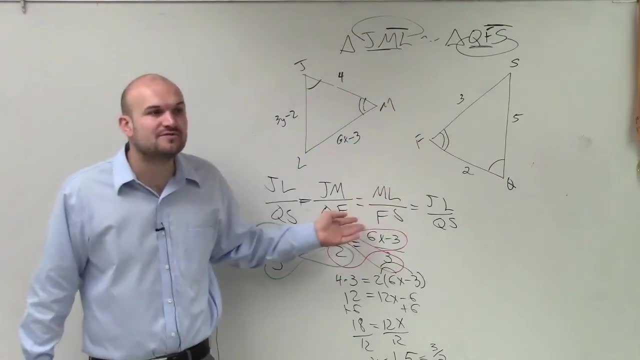 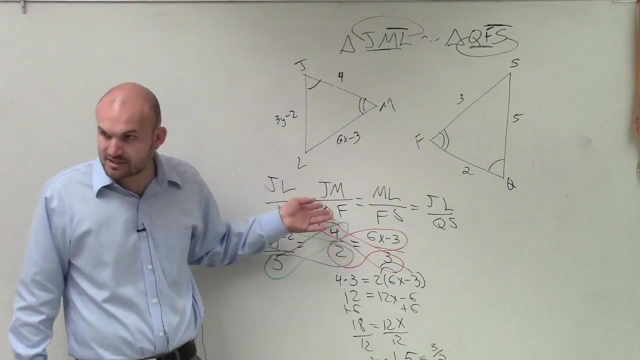 The difference is I have both of the values for JM and for QF, Right, I have both these values. There's no variables in this proportion, Right? Does everybody see? There's no variables in this proportion, So I can use it to help me solve for both of them. 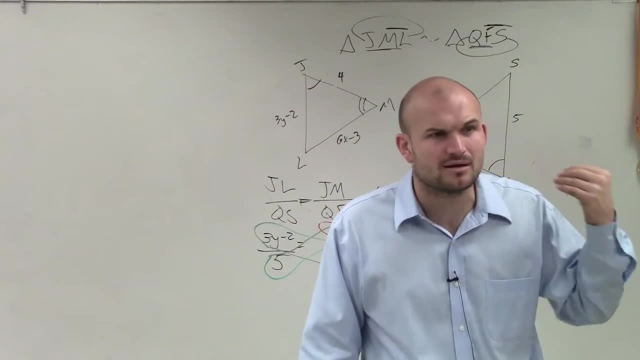 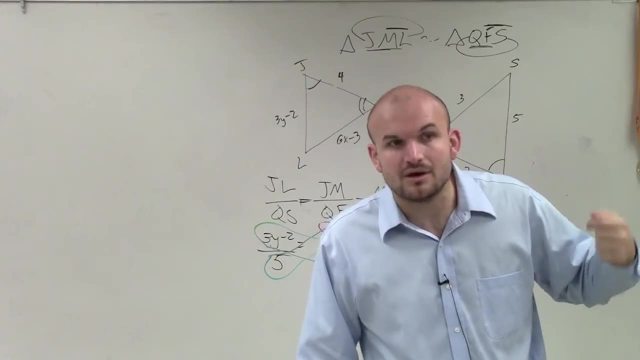 Taylor, I don't know why you just came in late. What? And the other one? Are you writing this down? OK, So if this is coming late, this is what you're going to want to know, because this is what you missed on. 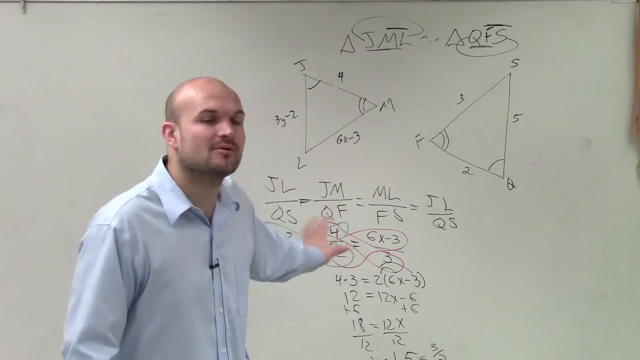 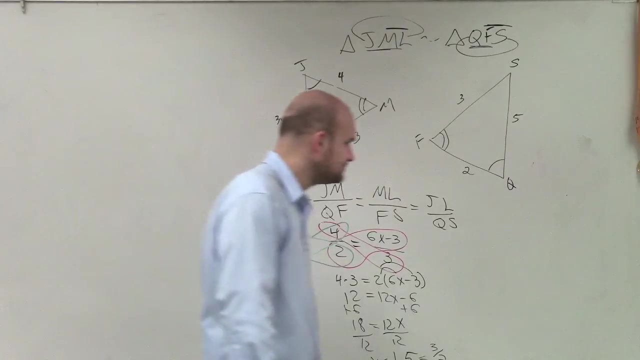 What I was saying, Taylor, is you missed this information, Right? So you're going to want to write this down, Because this is what you missed, Because this is what we're going over. So now, looking over here, let's go ahead and finish this up.